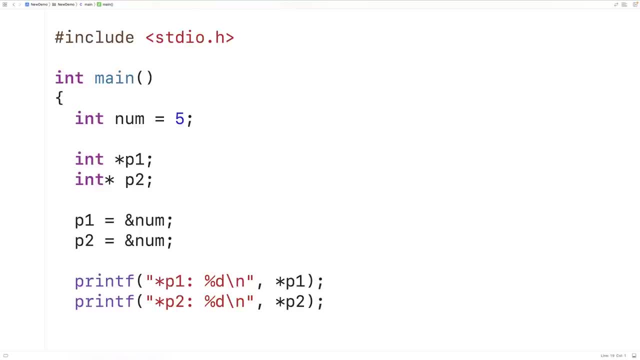 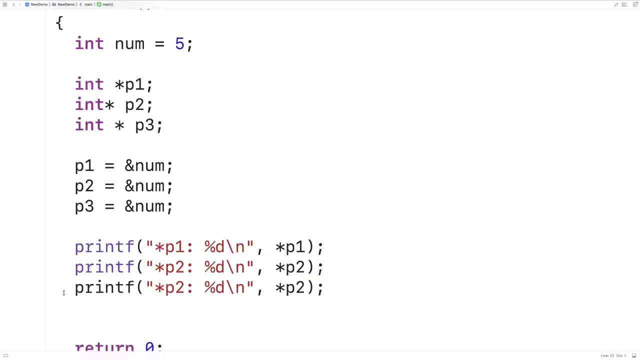 Instead and star p2 here, And if we save, compile and run this, we get that p2 points to the value 5 as well. So this way also works. We could also have this int space, star space, p3. And then here I could say p3 is equal to and num, And then down here I could print out p3. And this will also work. 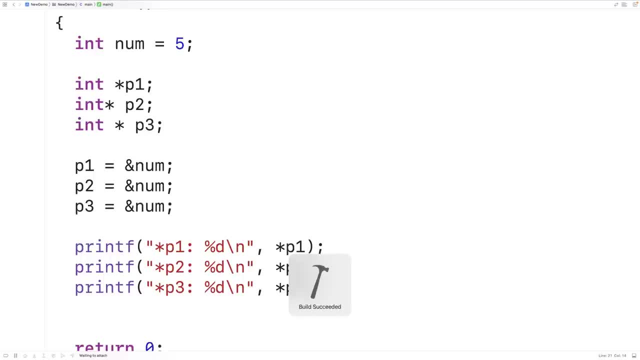 So we'll have p3 and p3. And if we save, compile and run it, we get that p3 points to the value 5 as well. So all of these approaches will allow us to declare a pointer to an int Of these three approaches. some people might say that this: 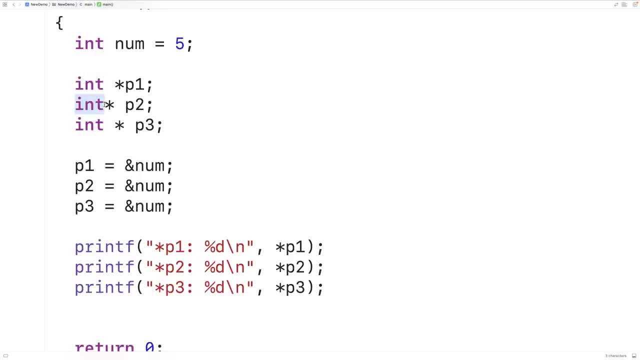 approach here is the clearest because it really expresses the type of the variable that we're declaring all together. We have the star right next to the int and it's a pointer to an int. This approach here tends to be the most confusing and that's very seldom used. 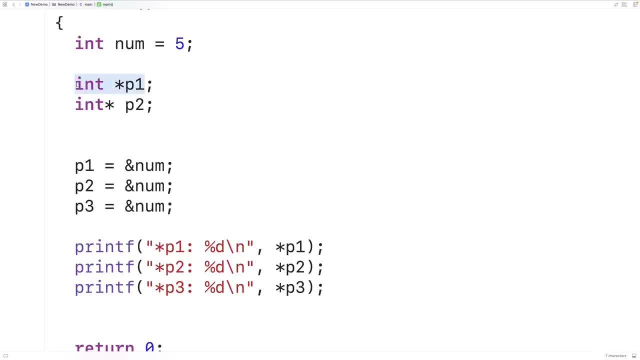 But oftentimes we'll see this first approach here used. Why is that So? to understand why it's used, let's try to declare multiple pointer variables with the same statement. So here we'll have p1, p2. And we'll delete the statement here. We'll also delete this here and this here, because we 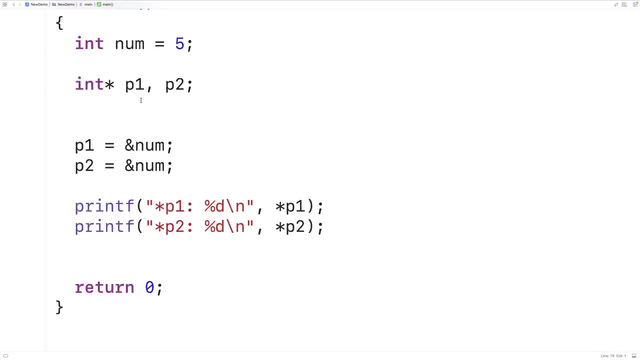 no longer have p3. So right now it looks like we should be declaring two pointers to an int. If we save, compile and run it, we get that p3 points to the value 5 as well, And if we save compile, 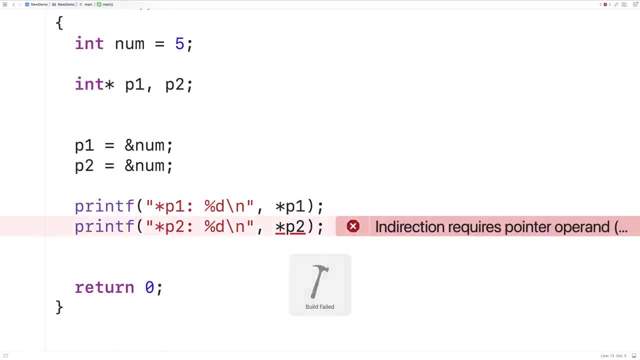 and run it. we get that p3 points to the value 5 as well. If we save, compile and run it, we get that p3 points to the value 5 as well. If we save, compile and run the program. we're going to get an error here, though It says indirection requires pointer. 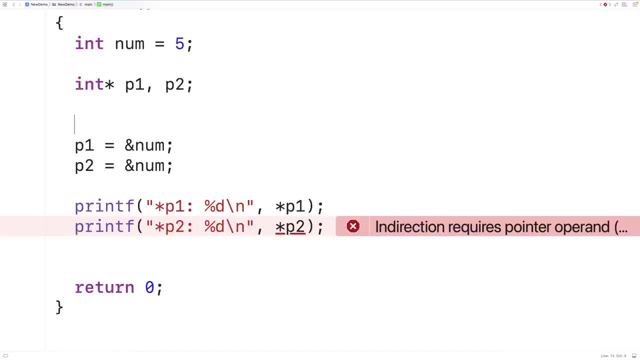 operand. So basically, the compiler is telling us that p2 is not a pointer. We could actually investigate this. Let's actually print out the size in bytes for a pointer to an int as well as the size in bytes for an int, And then we'll compare that. 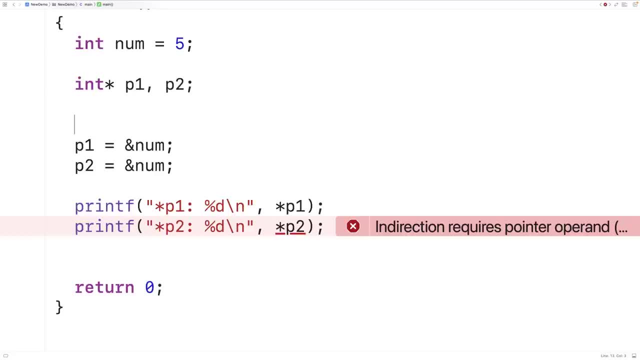 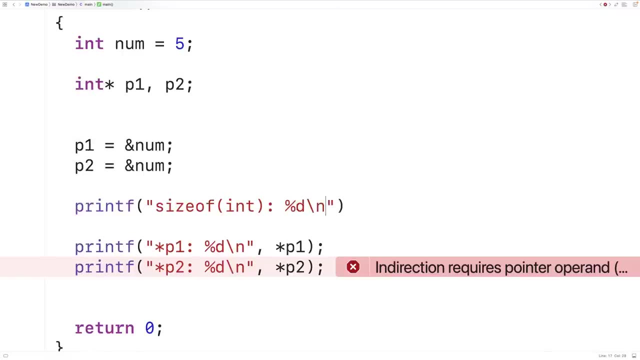 to the size in bytes for p1 and p2.. So here we'll have printf size of an int, colon %d backslash n, And we'll output the size of an int in bytes. We'll also print out the. 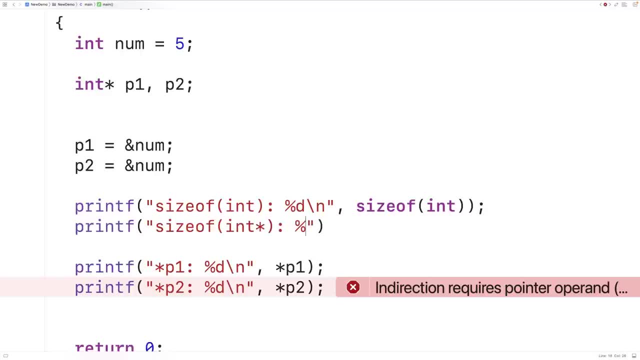 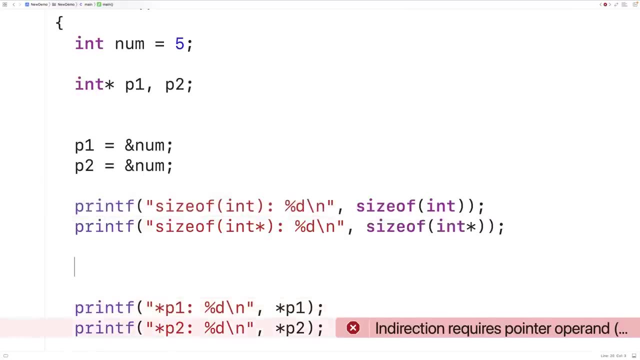 size of a pointer to an int in bytes with this statement here. So we'll have size of int star here. Then we'll print out the size of p1 and p2.. So we'll have printf size of p1, colon. 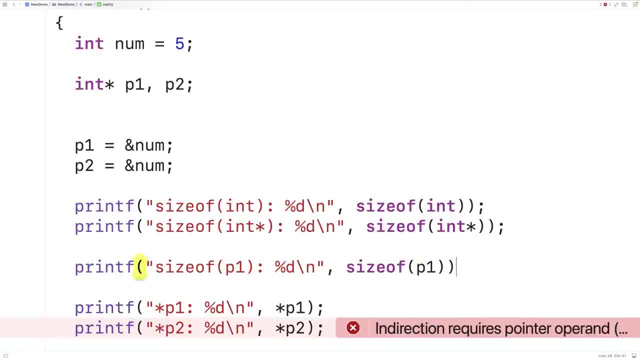 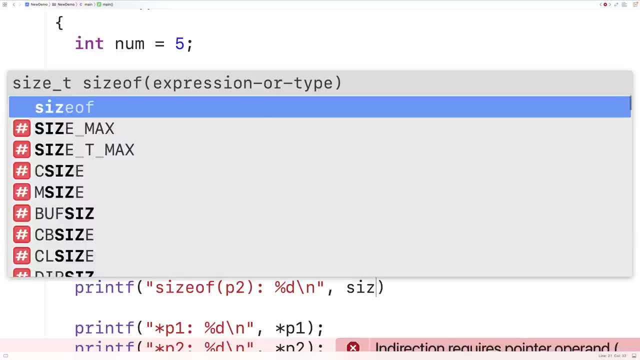 %d backslash n, And we'll output the size of p1.. Then we'll do the same thing with p2.. So printf: size of p2, colon %d backslash n- Size of p2.. And let's comment out this line here: 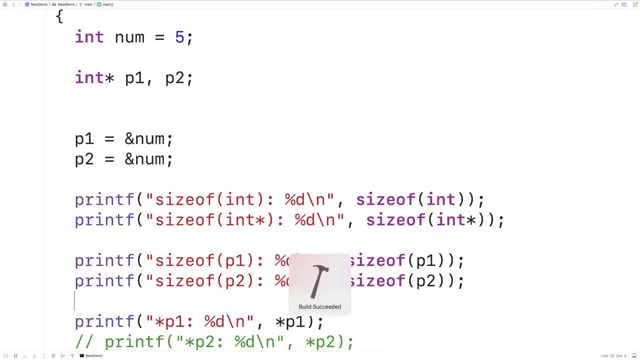 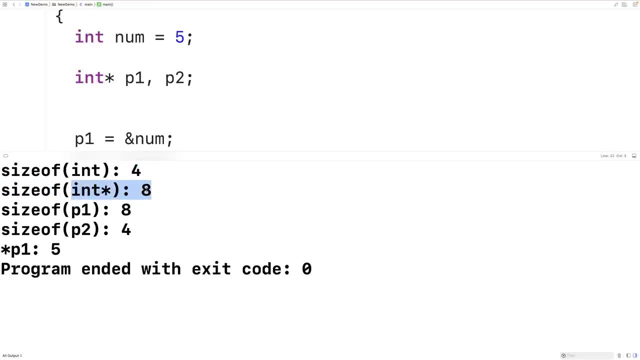 just so it compiles. So we'll save, compile and run the program And look at this. The size of an int is 4 bytes. The size of a pointer to an int is 8 bytes. The size of p1 is 8 bytes, So p1. 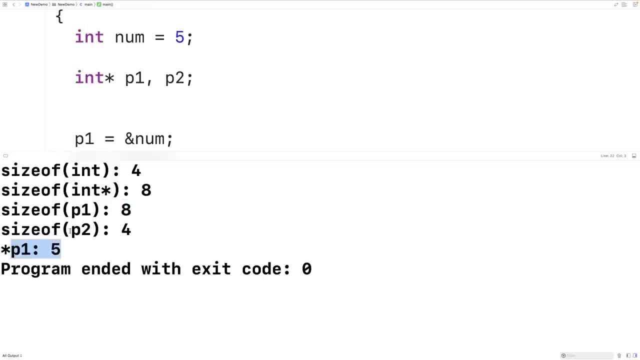 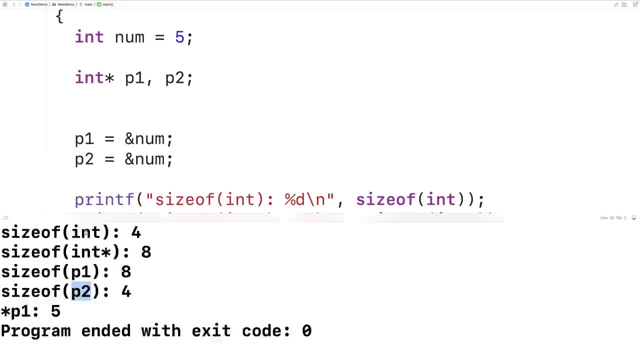 is a pointer to an int. That's why we can use it here like this: But p2 has the size 4 bytes. P2 is actually an int. It's not a pointer to an int. That's why we get this compilation error when. 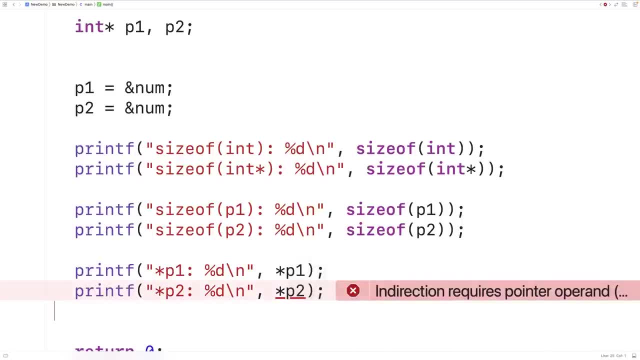 we try to use it like a pointer and dereference it. So what's really happening here is that, because this star is here, p1 is being declared as a pointer to an int, but p2 is being declared as an int. If we wanted to declare p2 as a pointer to an int, we would have to put a star over here. 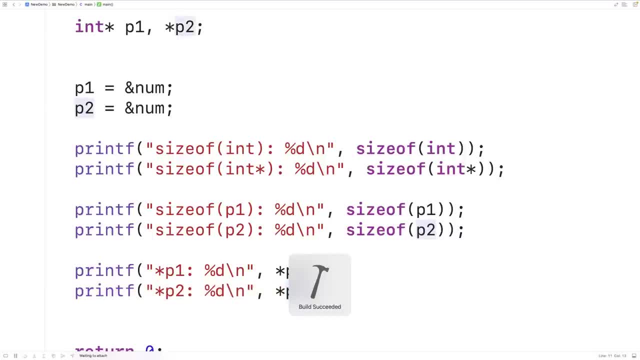 like this: If we now save, compile and run it, it's going to work and p2 does again point to the value 5.. Now we could put the star here: save, compile and run it, and this will also work. 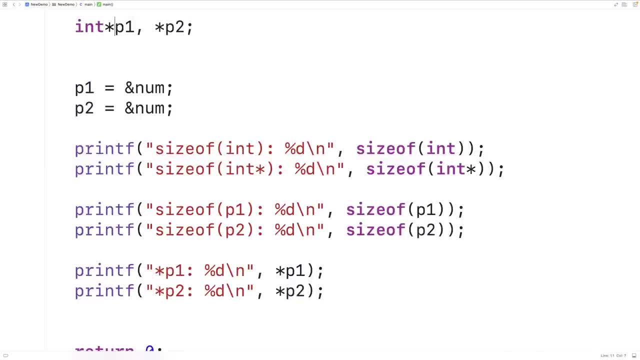 but it seems to make more sense to have the star next to each variable name. So that's the approach you tend to see used in practice, because it makes it clear that both of these variables are a pointer to an int. Now, because of this potential for confusion, 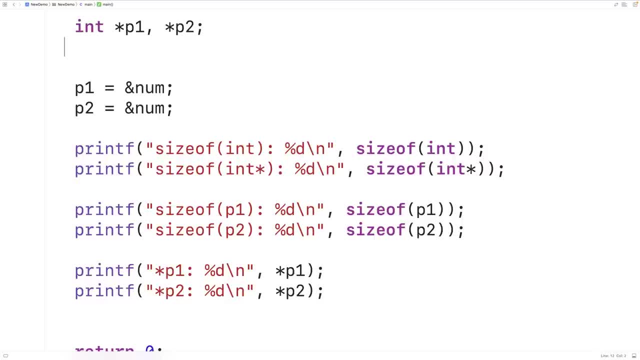 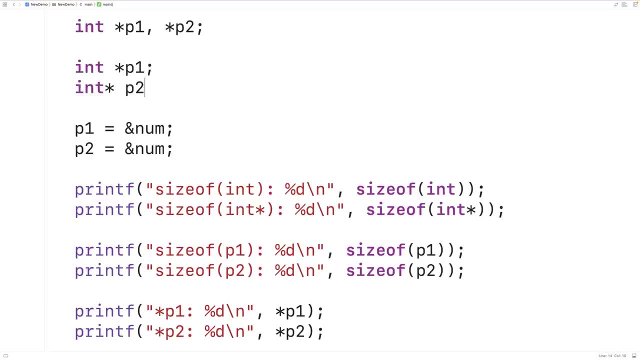 we may actually want to limit our variable declarations to one variable per line, like this: int star p1 or int star p2.. Now the reason why I wanted to make this video is that this approach here could be confusing if you're not familiar with how pointer variable declarations work.